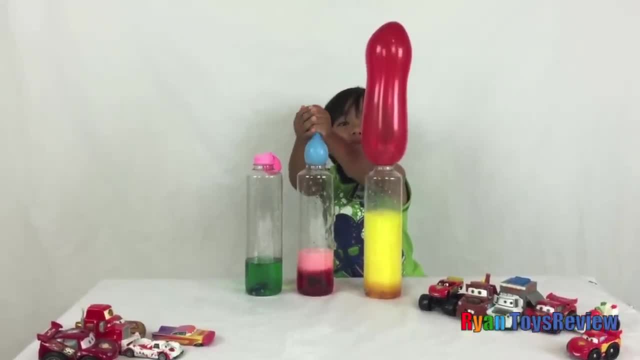 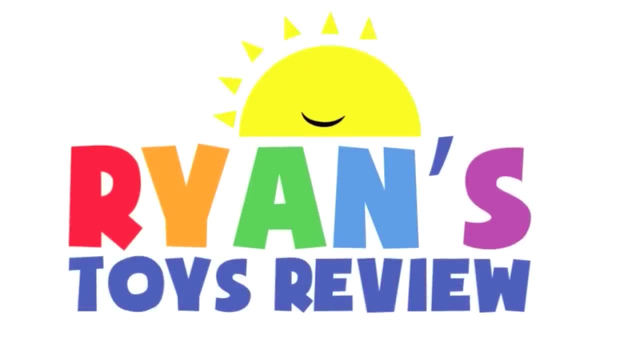 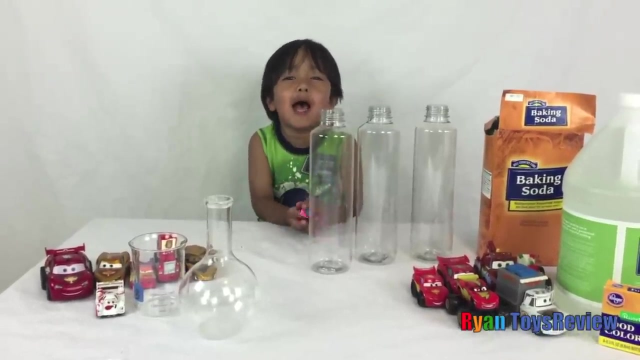 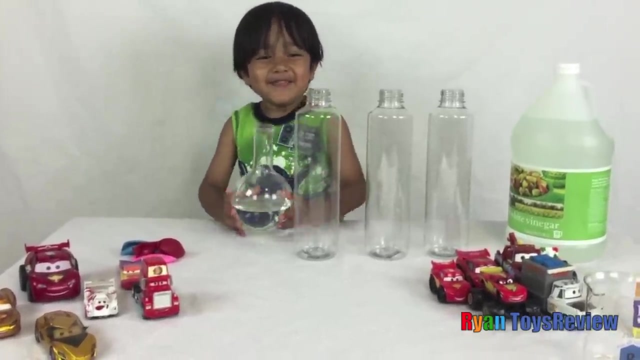 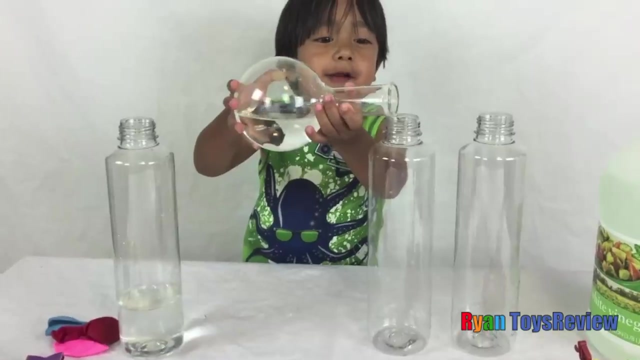 Hey Ryan, Hi Mommy, What are we going to do today? We're going to blow the balloon up. That's right. Let's fill the empty bottle with vinegar. Now, the second one. Next, I'm going to add food coloring. 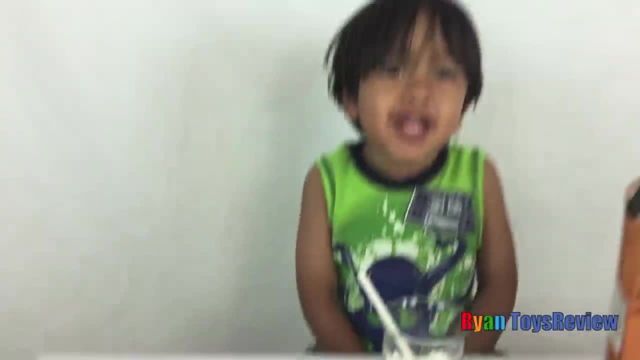 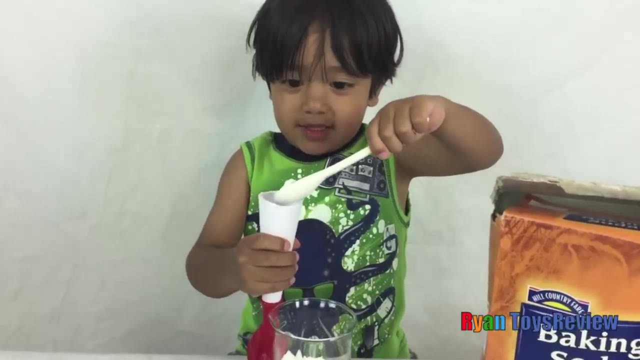 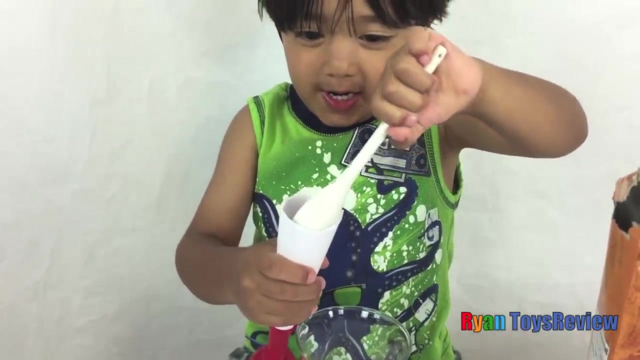 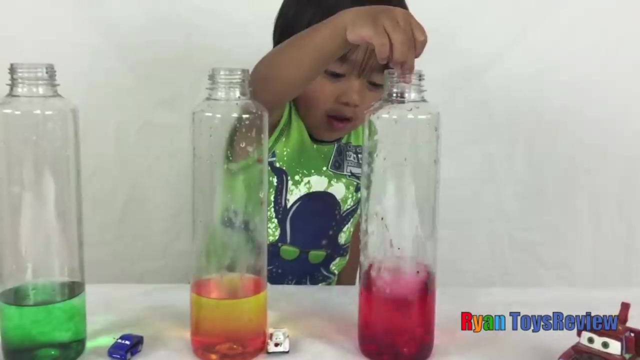 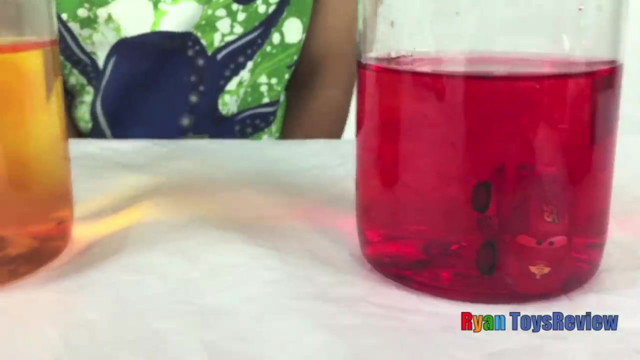 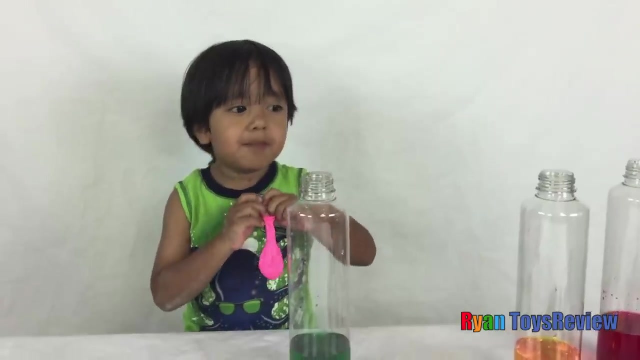 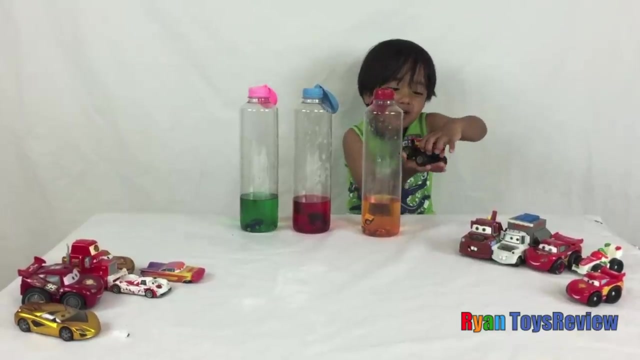 Using the funnel, I'm going to fill the balloon with baking soda- The big one. I'm going to put the micro drifter inside for fun. Now I'm going to put the balloon over the bottle. Disney Cars, are you ready to enjoy the show? 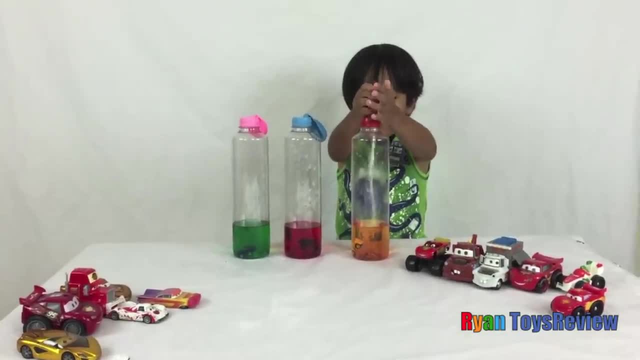 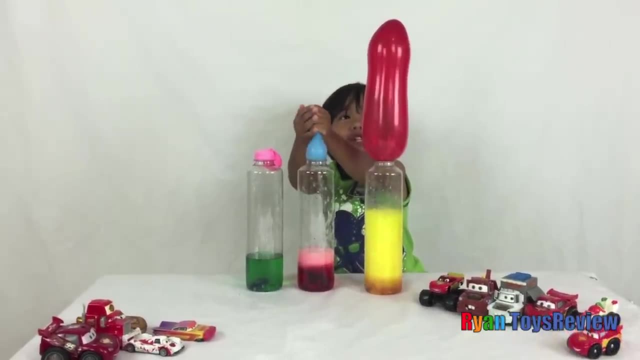 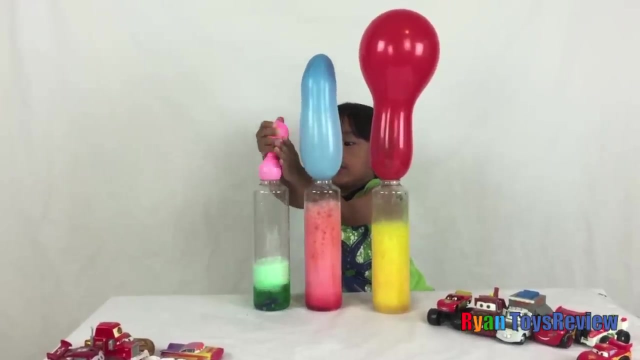 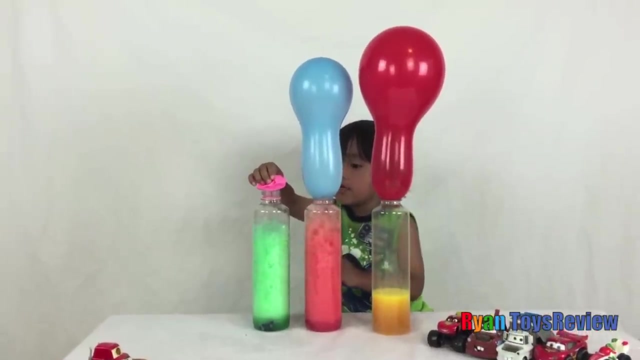 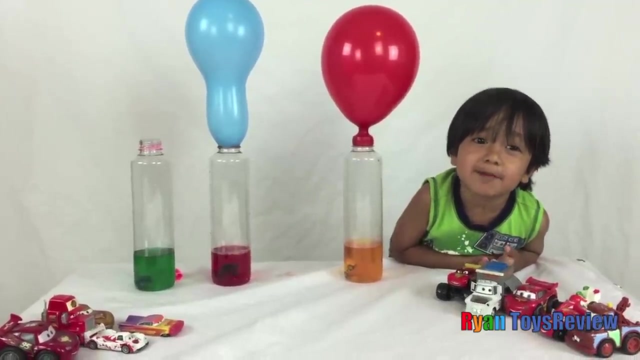 Yeah, I want to. Whoa, It's blowing my face again. Whoa, Oh, Oh no. Hahaha, Oh no, It's going to go up, It's okay. Do you want more Air Made by Ryan? Look, This is spectacular. 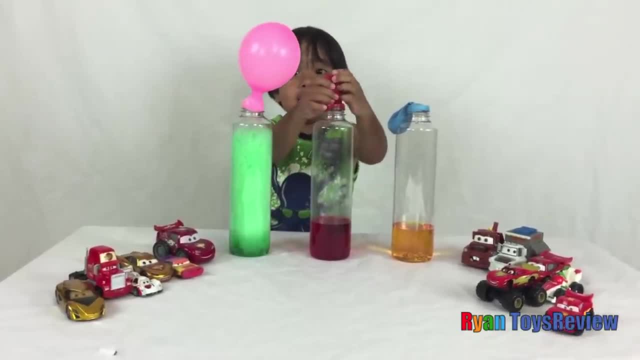 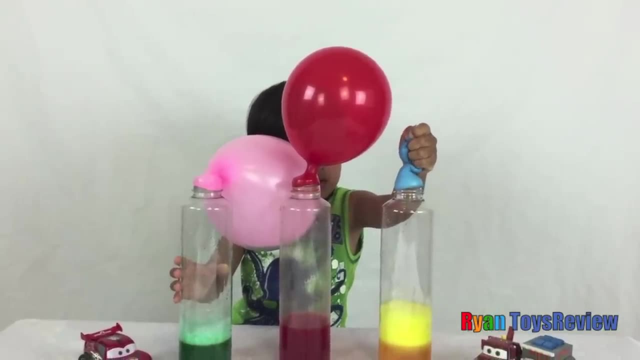 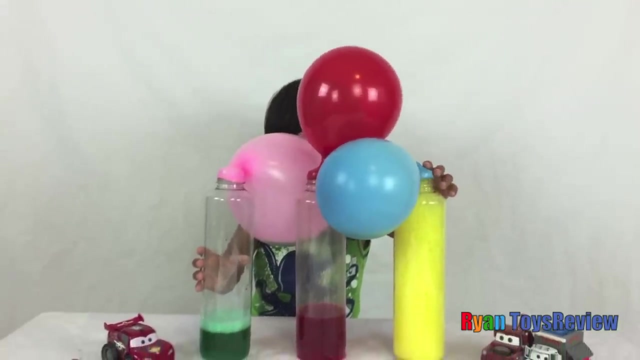 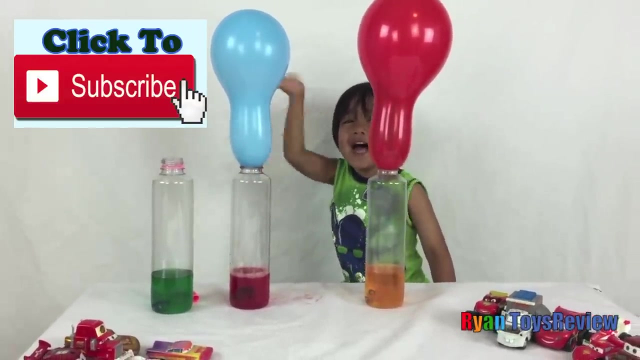 Oh, It's so big, Ryan, I can't even see you. It's another balloon, Hahaha. If you like this video, please subscribe. Bye, Don't forget to subscribe. See you later, Bye. Whoa, Do you want more Air Made by Ryan. 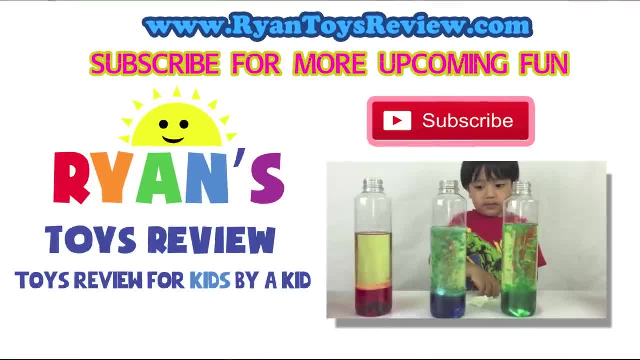